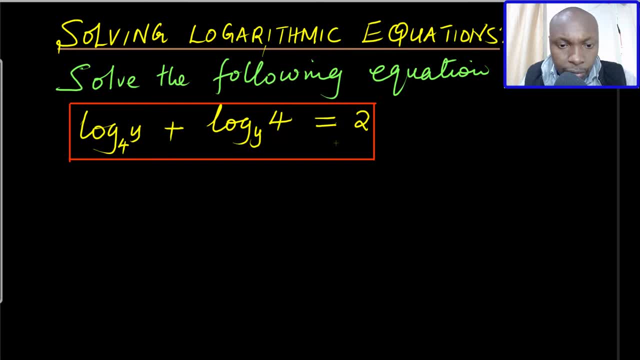 this question. A quick look at this question, you notice that we have bases that are different. The first one log of y to the base of four, this one to the base of four, then the next one is to the base of y. Now, you cannot solve this one easily unless you change all the. 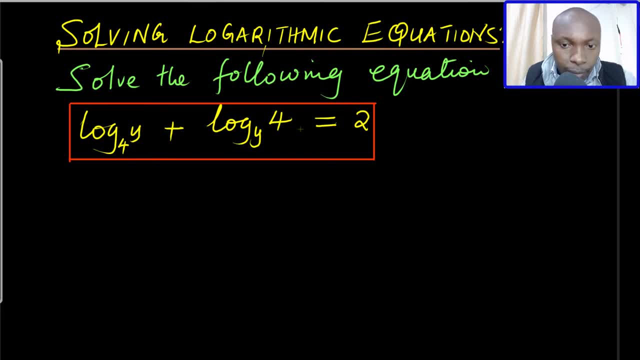 bases to be uniform. So in this case, I'm going to change all of them to be to the base of y. So therefore, I'll require- I'll be required- to change log of y to the base of four to be log of four to the base of y. 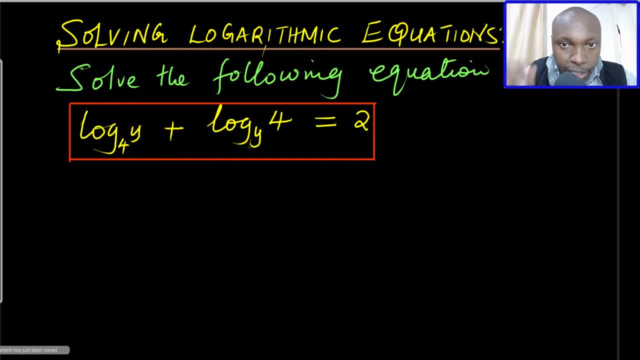 So that the bases will be the same and in this case, the bases will be y. Now, to do this, these are rules that you need to know- the change of the base rule. So, change of the base rule. what does this state? In case you're given, let's say, log of a to the base of b. 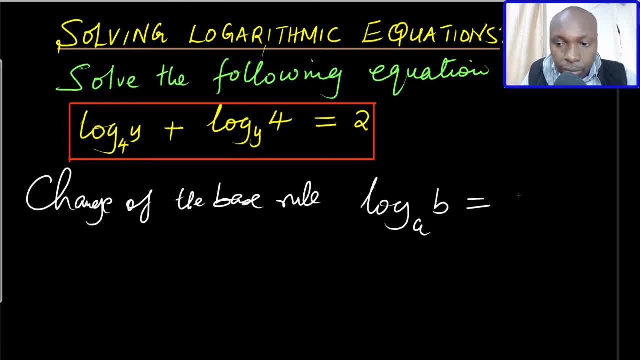 and you want to change so that now the base will be b and not a. This will be given by the inverse of log of um. now the base will be b and that will be one divided by log of a to the base of b. So that is what we're going to apply. so in this case, load of um. 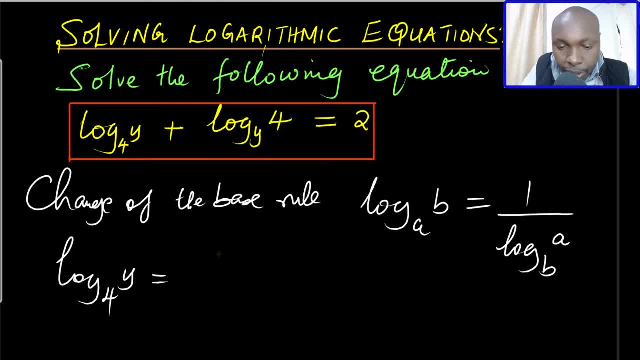 y to the base of four. If we want to change this base, I'll have it as y. And so, in this case, log of y to the base of four. You want to change this base? I'll have it as one. How to do So? first, we're going to be quarantined here, So in this case you can forward this. 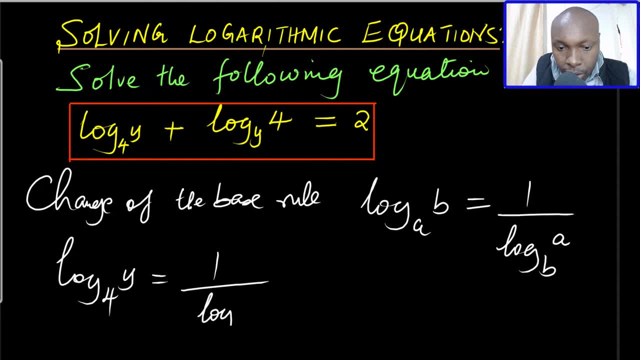 base to e, and that's what it says. So first we drive this. So this is the first zijn to. It is 1, divided by log of 4 to the base of y. So now you can see this one will be to the base of y and I'll have the other one to the. 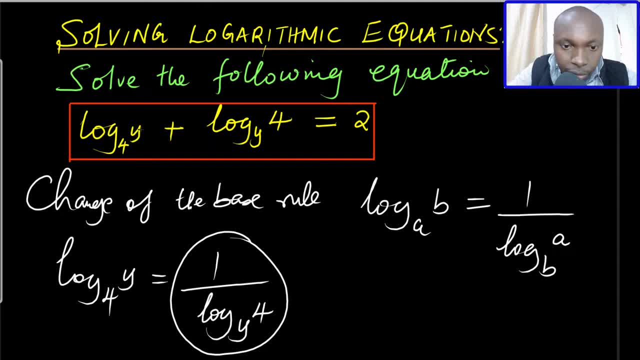 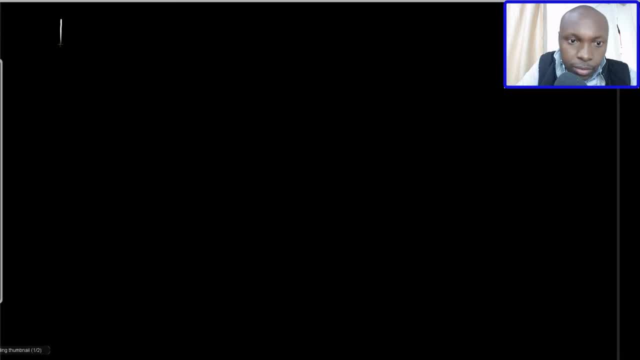 base of y. Now, having that now, instead of having now log of y to the base of 4, I will write it as 1 divided by. so this will be 1 divided by log of 4 to the base of y. 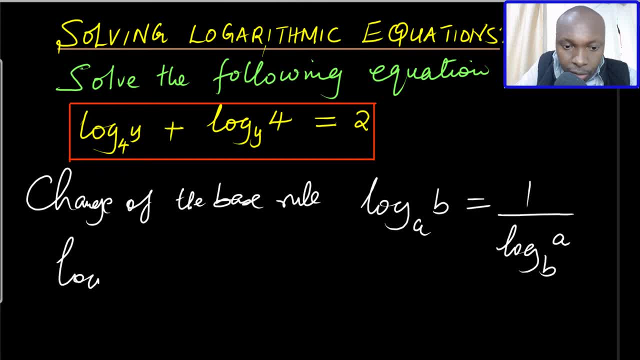 So that is what you're going to apply. So in this case, log of y to the base of four. we want to change this base. I'll have it as one. I don't want to change this base. So 1 divided by log of 4 to the base of y. 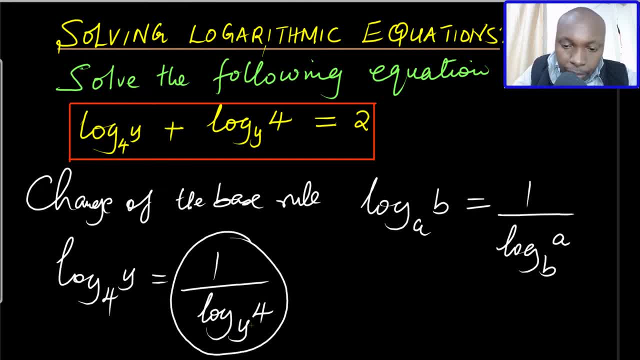 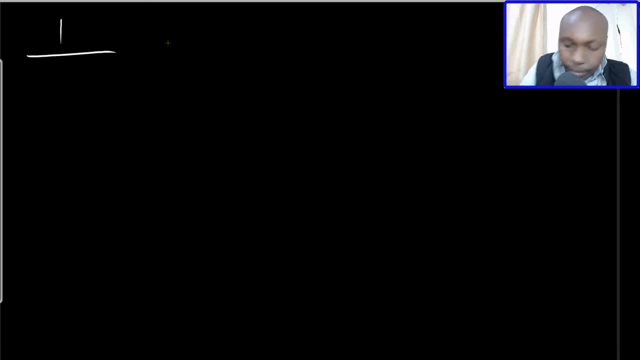 So now you can see, this one will be the base of y and I'll have the other one to the base of y. Now, having that now, instead of having now log of y to the base of 4, I will write it as 1 divided by. so this will be 1 divided by log of 4 to the base of y. 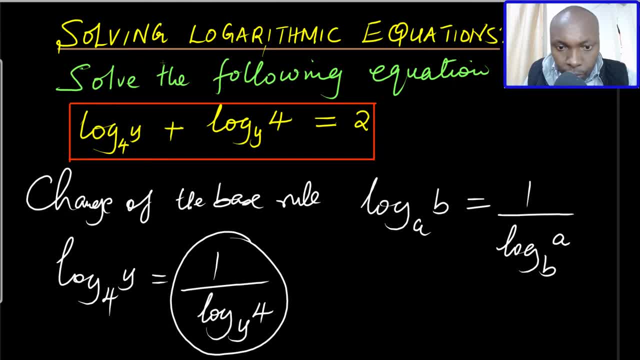 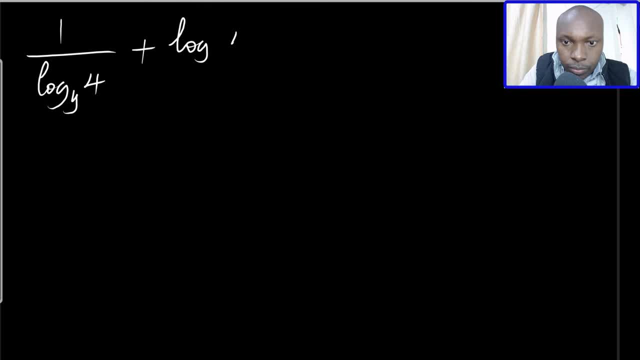 Then plus, the other one is log of 4 to the base of y, log of 4 to the base of y. This one should be equated to 2.. Now, by doing that, now I'll be able to solve, since the bases are the same. 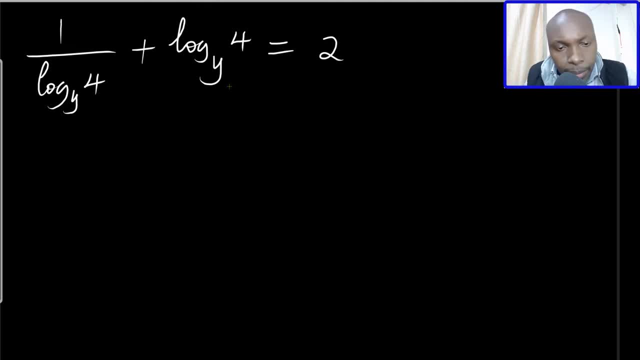 The base is y, the uniform now. Now, from this step, the next thing that we're going to do, you can let log of 4 to the base of y be a letter. let's say m. I'll leave that one to be m. 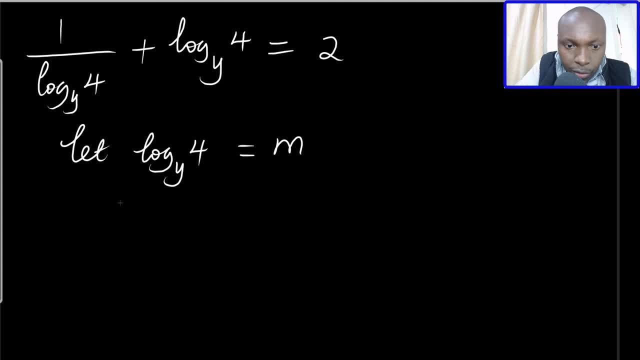 That is m. Therefore, instead of 1 divided by log of 4 to the base of y, you shall have 1 divided by m. Okay, So 1 divided by m plus m, this one should be equals to 2.. 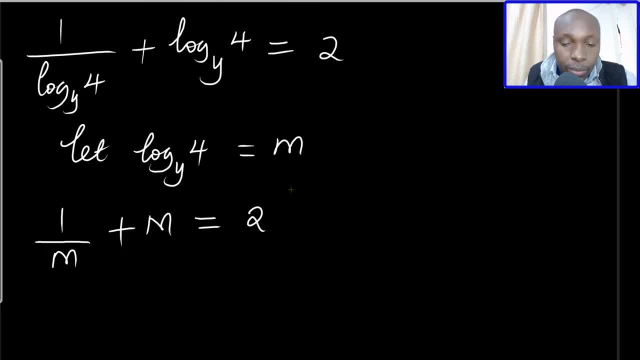 Now you can see you're simplifying the equation. it is becoming simpler now to work with, Now having that if I multiply each term by m, if I multiply each term by m like this, I get m multiplied by 1, divided by m, plus each term. 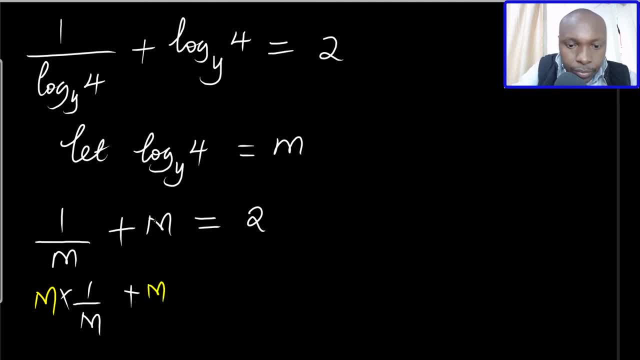 Each term to be multiplied by m times m is equals to, then this one will be 2 multiplied by m. Now, if I do that, if I do that, this one I'll have, this one I'll have. for this one, I'll. 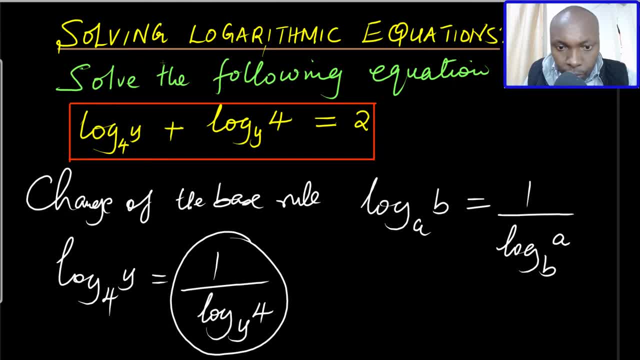 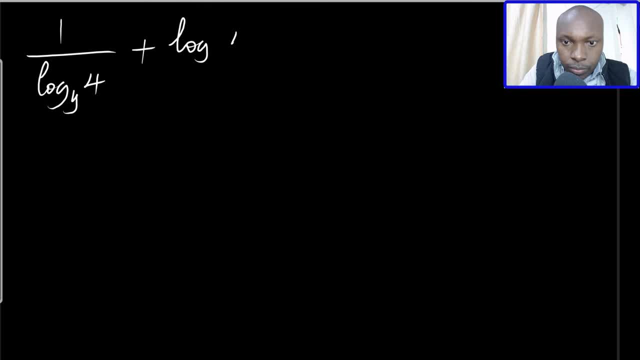 Then plus, the other one is log of 4 to the base of y, log of 4 to the base of y. This one should be equated to 2.. Now, by doing that, now I'll be able to solve, since the bases are the same. 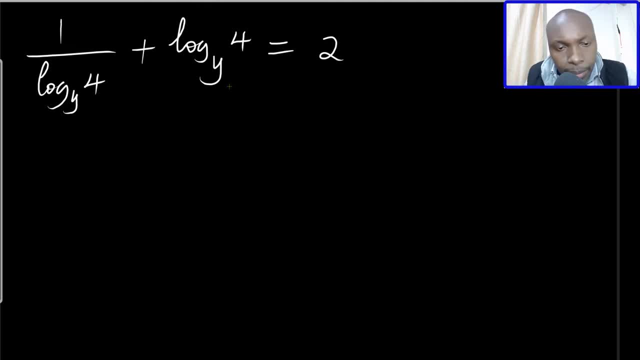 The base is y, the uniform now. Now, from this step, the next thing that we're going to do, you can let log of 4 to the base of y be a letter. let's say m. I'll leave that one to be m. 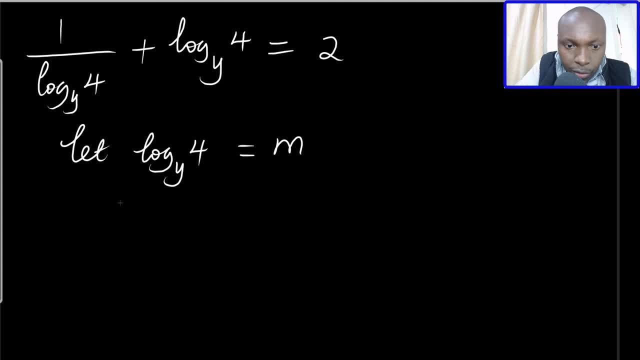 That is m. Therefore, instead of 1 divided by log of 4 to the base of y, you shall have 1 divided by m. Okay, So 1 divided by m plus m, this one should be equals to 2.. 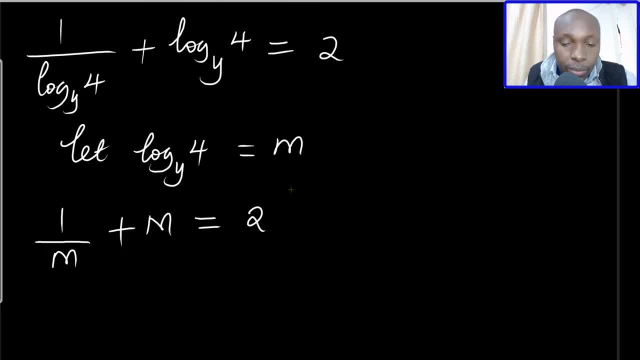 Now you can see you're simplifying the equation. it is becoming simpler now to work with, Now having that if I multiply each term by m, if I multiply each term by m like this, I get m multiplied by 1, divided by m, plus each term. 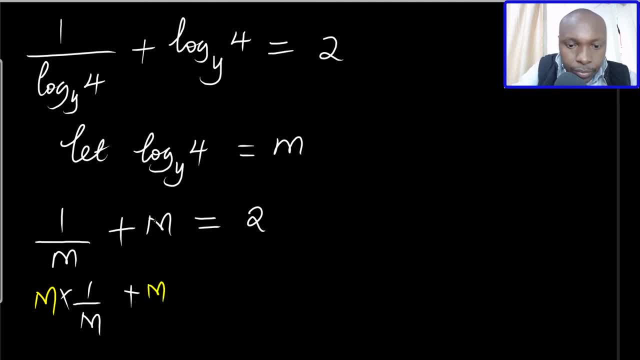 Each term to be multiplied by m times m is equals to, then this one will be 2 multiplied by m. Now, if I do that, if I do that, this one I'll have, this one I'll have. for this one, I'll. 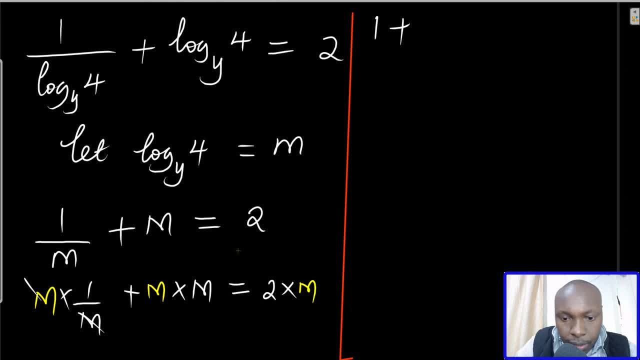 have 1.. Okay, So 1 divided by m plus m squared is equals to 2m. Now organizing this one, because you can see, this one will form a quadratic equation. I'll have m squared minus 2m plus 1 is equals to 0.. 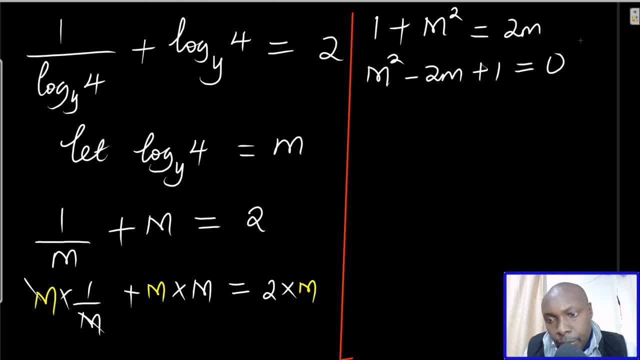 So using the initiative method to solve for m use the factorization would work very well here. So look for two numbers: That is 1 and the sum is negative 2.. So I'll have m squared. minus m, minus m, that will be minus 2m. plus 1 is equals to 0.. 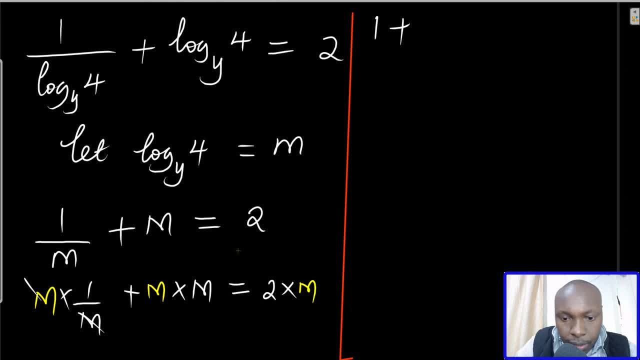 have 1.. Okay, So 1 divided by m plus m squared is equals to 2m. Now organizing this one, because you can see, this one will form a quadratic equation. I'll have m squared minus 2m plus 1 is equals to 0.. 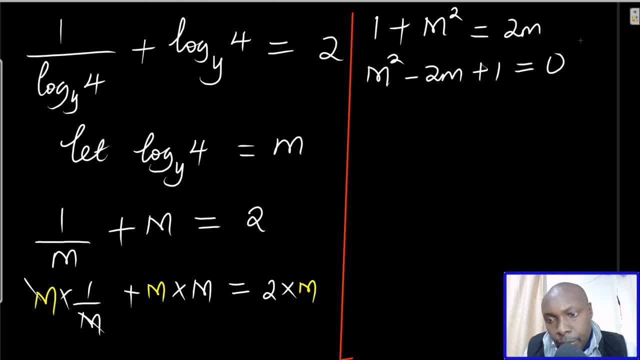 So using the initiative method to solve for m use the factorization would work very well here. So look for two numbers: That is 1 and the sum is negative 2.. So I'll have m squared. minus m, minus m, that will be minus 2m. plus 1 is equals to 0.. 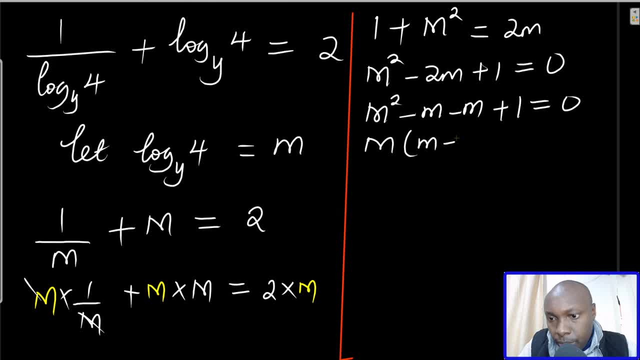 Factorizing, you get m minus 1, then minus 1, this one is m minus 1, is equals to 0. So therefore, m minus 1 multiplied by 2m, So m minus 1 multiplied by m minus 1.. 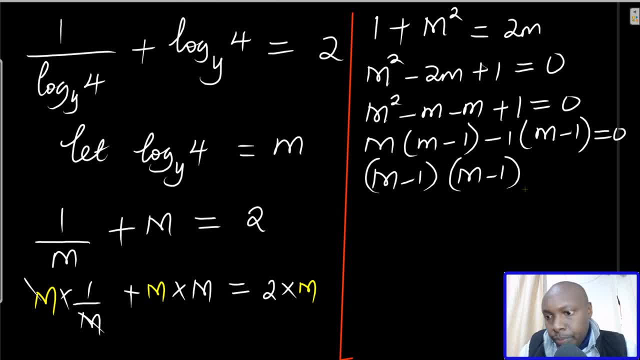 So it will be ok. and this one should be equal to 0.. So you can see, both of them are similar. m minus 1 is equals to 0, and m minus 1 is equals to 0. So you shall have m to be equated to 1.. 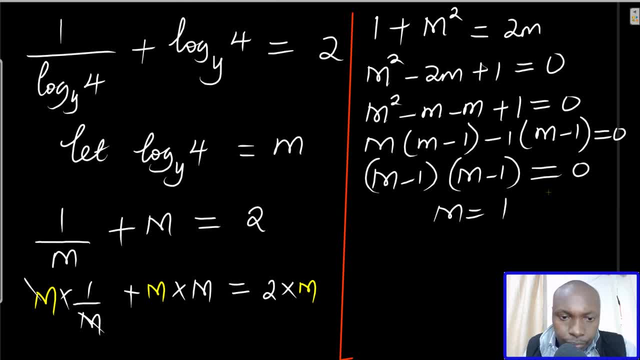 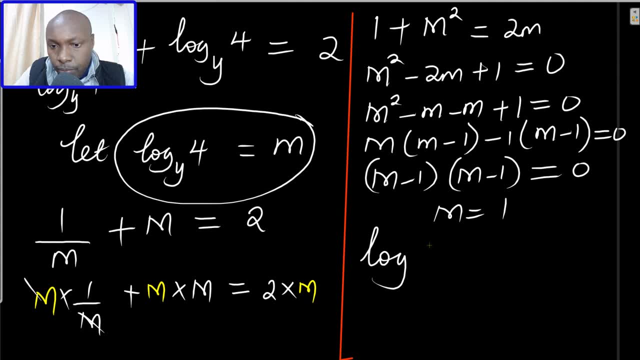 Now, after getting m, now you can recall, but you have this- that log log of u equals m. Okay, So we can use this one. So this is our first term. We're going to use our first term, w. 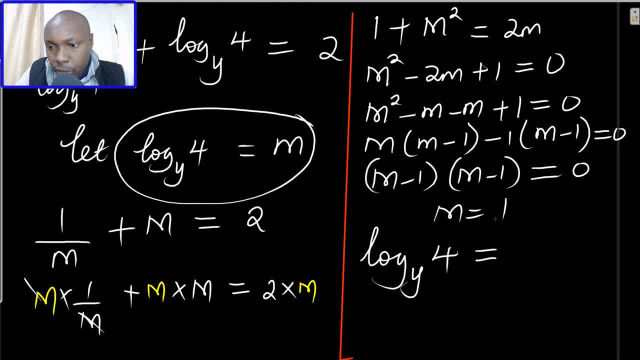 y log of 4 to the base of y is equal to m, m is 1.. Now, from here, now you can get your m easily. Why, Since this one is written in logarithmic notation, if you want to write this one in index notation? 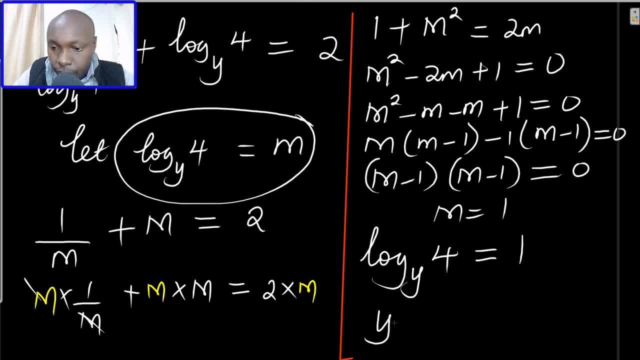 you shall just do it like this. You take y raised to power, 1 should be equal to 4.. So you are just writing: this one is in logarithmic notation. now you want to write it in index notation. This one is index notation. 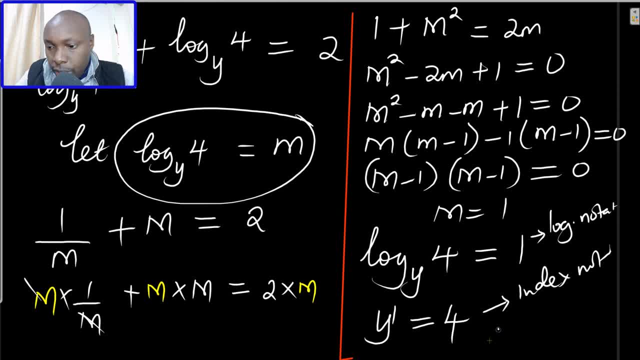 So you get y raised to power: 1 is equal to 4 and therefore y is equal to 4.. As simple as that.